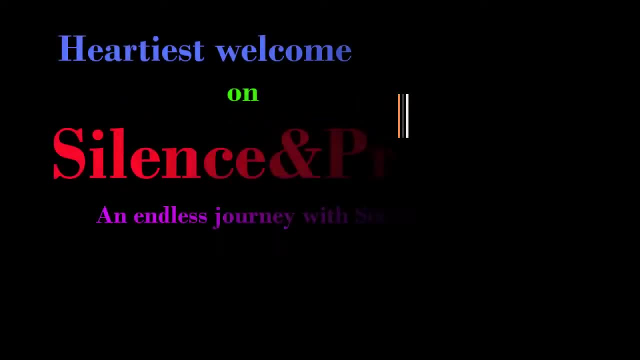 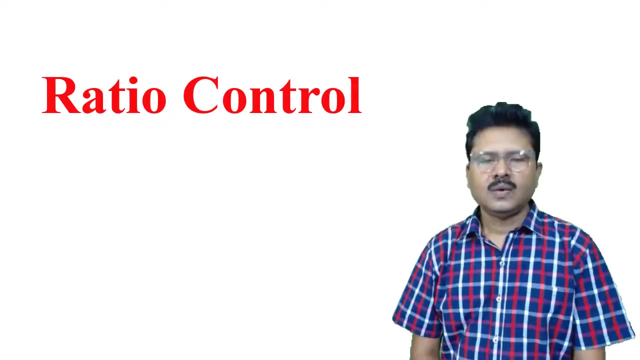 Welcome on this tutorial. Wish all your well. In this tutorial we are going to discuss about ratio control system. Ratio control system is a particular control technique whose objective is to maintain a particular ratio between two variables without any external disturbances. Ratio control system is a special type of feedforward control system. This ratio control 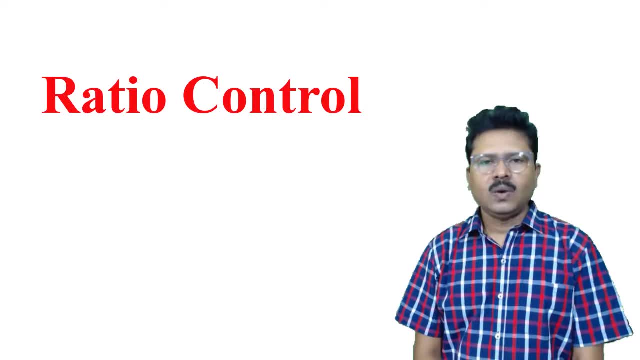 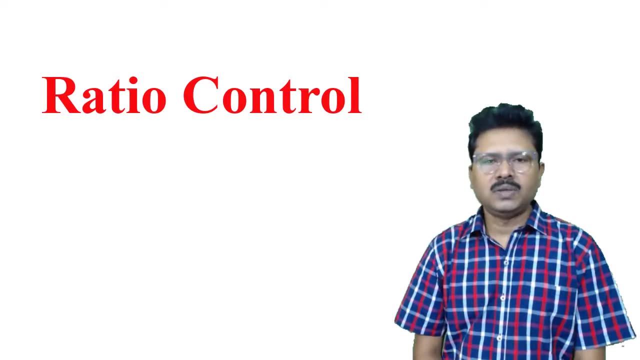 system is mainly used in chemical process plant where more than one variable should mix in a specific ratio. The stream whose flow is measured but cannot be controlled is termed as wild flow, or wild stream or master flow. The other flow which is measured and controlled is termed as controlled flow. Ratio control system manipulates the controlled. 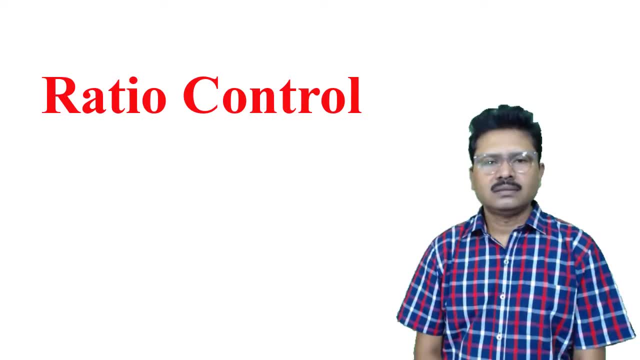 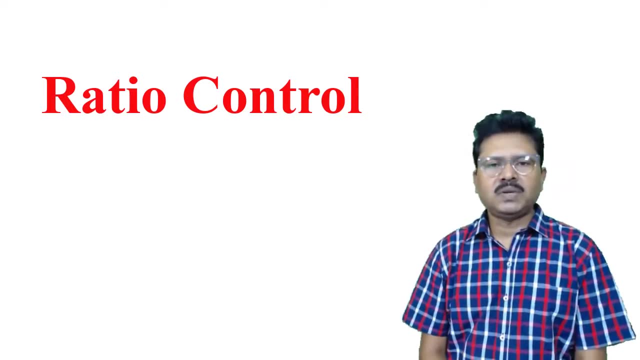 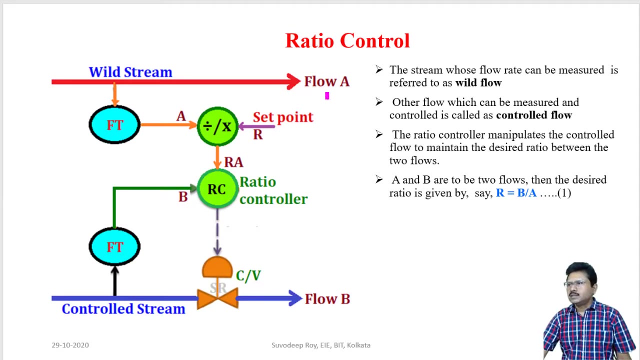 flow to maintain desired ratio between two flows. I am entering into the discussion of ratio control system in details. Please subscribe the channel. It will help me to improve it. This is a particular diagram which describes the ratio control system. Two flows are here. 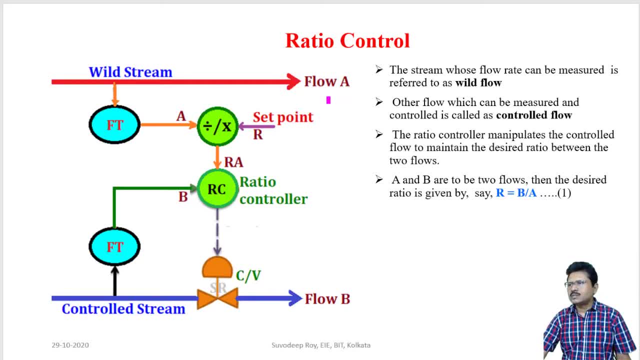 flow A and flow B. Target of this control system is to maintain a specific ratio between these two flow A and B. Flow A is measured by this flow transmitter. Flow B is measured by this flow transmitter. Flow B may be termed as controlled stream. Flow A is measured and with respect to value. 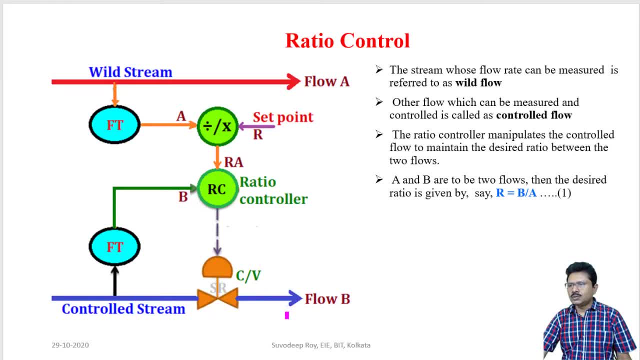 of this flow A, flow B is controlled. This Ft transmitter gives the flow of A, which is the input of this converter. This converter might be a divider or might be a multiplier. This is the ratio R, which is the input of this converter. This is the ratio R which. 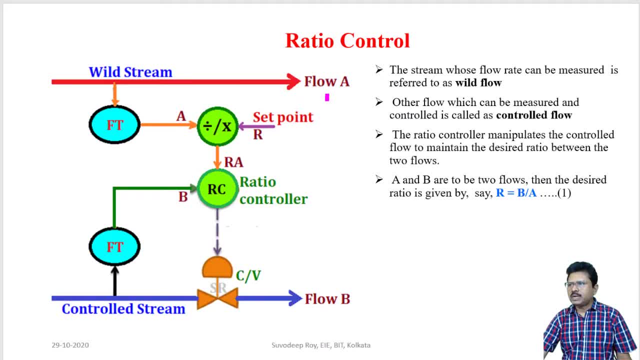 is the set point at which there will be a ratio between flow A and flow B. Say, the ratio is B by A, where B is controlled flow and A is wild flow. Now, from this relation, R is equal to B by A. Value of B will be R. This is value of flow A. This is the set point. 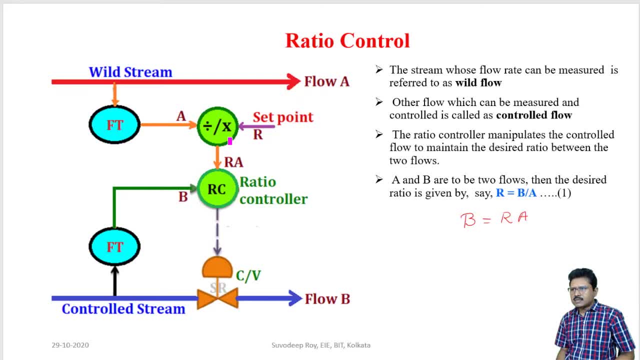 at which the ratio needed to maintain, and this acts as a multiplier. It will Tw r and a. ultimately, it will produce a value which is r a. now this r a is the set point of this ratio controller. from this relation, to maintain a ratio, b by a, the value of b should be r into a. 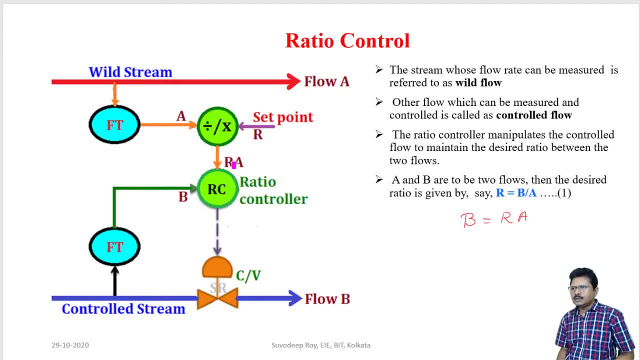 so this should be value of b. this is the set point for this ratio controller. now, flow b is measured by using this flow transmitter. here the signal is flow b and this is the set point, which is r into a means the flow b should be equal to r into a if there is any difference between these two signal. 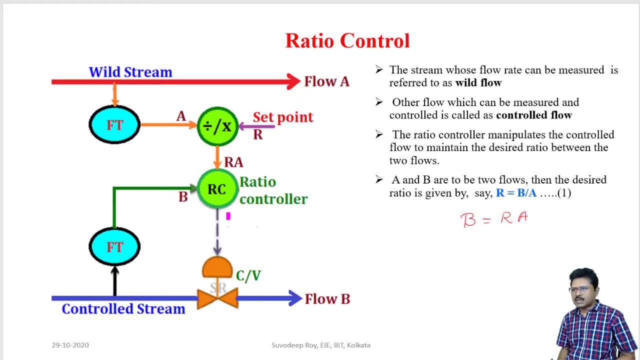 this ratio controller will produce a particular output. that output will operate the control valve to maintain the flow at a desired value so that the ratio between flow a and flow b should be equal to r. as an example, i am considering ammonia plant in ammonia plant for production of ammonia. 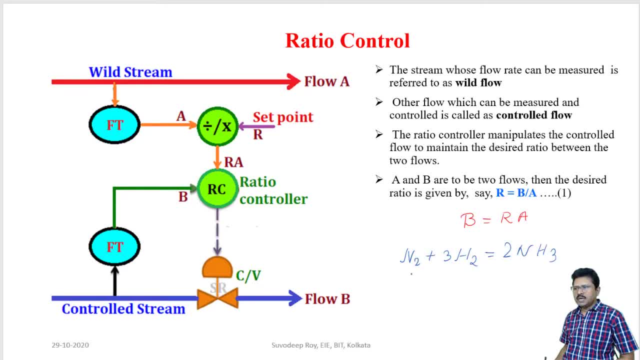 three unit of hydrogen should be mixed with one unit of nitrogen to produce ammonia. so nitrogen and hydrogen will be mixed here at a ratio of 1 is to 3. if we say hydrogen is flow b and nitrogen is flow a, then value of ratio b is equal to r and r is equal to r. so this ratio controller will be. 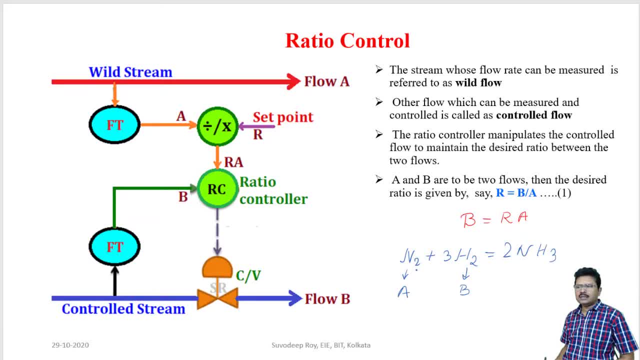 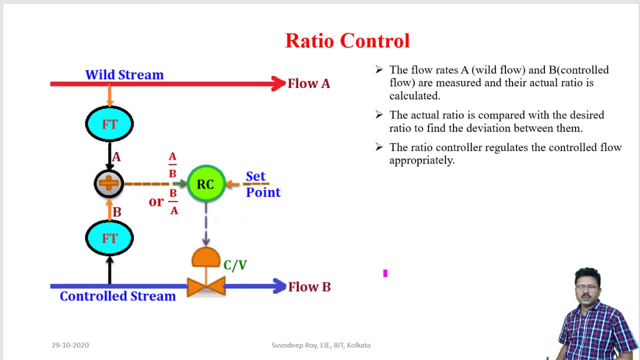 equal to r is equal to 3. divided by 1, that is 3. so the value of r for the case of ammonia production should be 3. this is another figure to explain ratio control system: flow a and flow b. flow a is wild flow. flow b is controlled flow. flow a is measured by this flow transmitter. so this is the 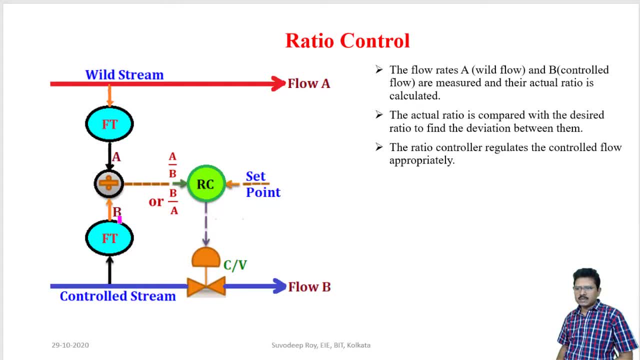 flow a signal. flow b is measured by this flow transmitter and this is flow b. here this is ratio calculator. it will calculate ratio between a and b. ultimately it will produce the exact ratio. here this is the measured variable or feedback signal for this ratio controller. set point will be given here according to the desired value. 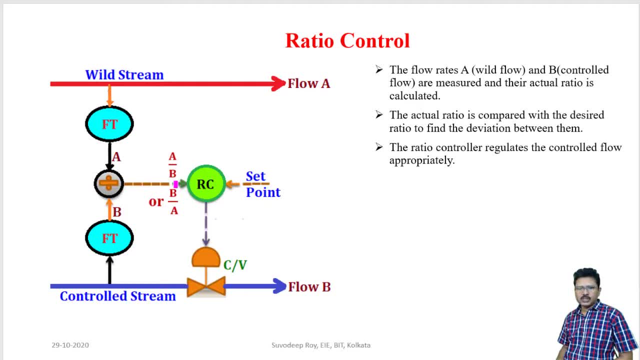 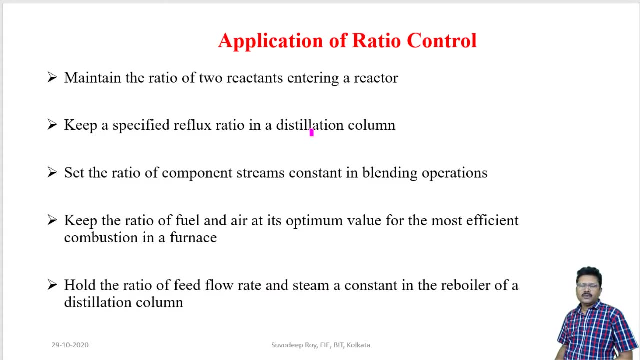 this controller will compare the set point with this ratio value and if there is any difference between these two, then it will produce a particular signal. this will operate the control valve which will control the flow b, ultimately to maintain ratio between flow a and flow b. few examples of 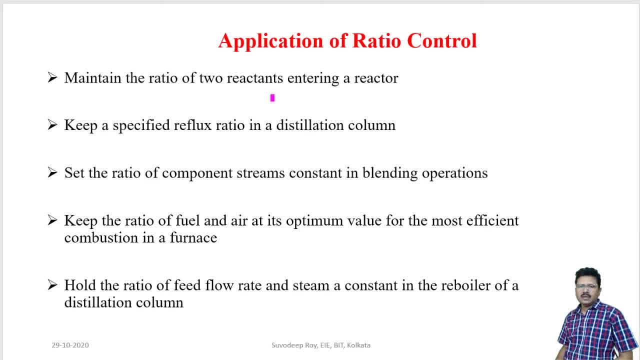 ratio control systems are used. it is used to maintain ratio of two reactants entering into the reactor. just like the example we have already given for the case of ammonia plant, the ratio control system is used to keep a specified reflex ratio in a distillation column. ratio control system is to set the ratio of component streams constant in blending operation. 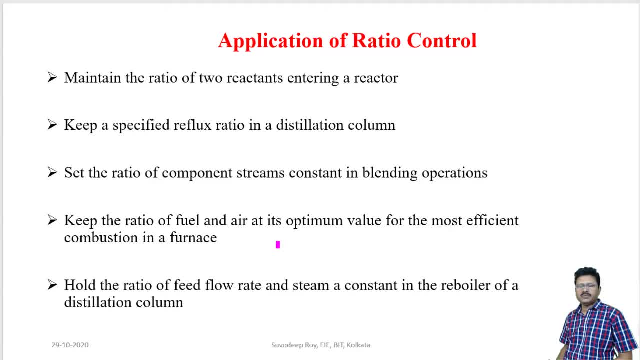 the ratio control system is used to maintain the ratio between fuel and air at its optimum value for the most efficient combustion. in the furnace, ratio control system is used to hold the ratio of feed flow rate and steam a constant in the re-boiler of a distillation column. so these 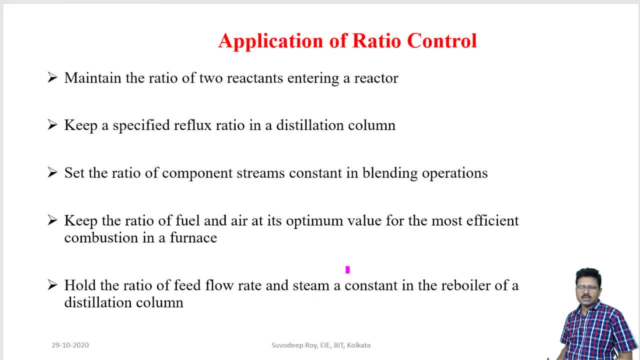 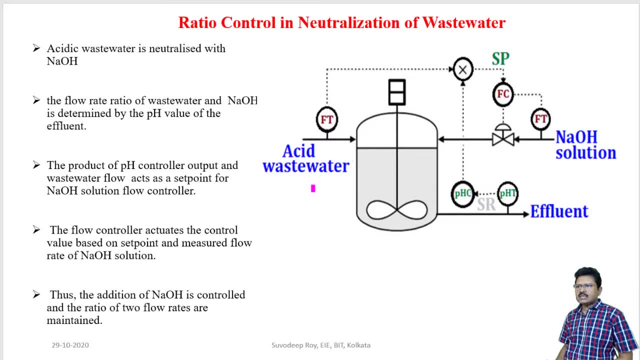 are the different examples where ratio control systems are used. this is one of the example where ratio control is used in neutralization of wastewater. acidic wastewater is neutralized with sodium hydroxide. as sodium hydroxide is basic in nature, the flow rate ratio of wastewater and sodium hydroxide is determined by the phd. 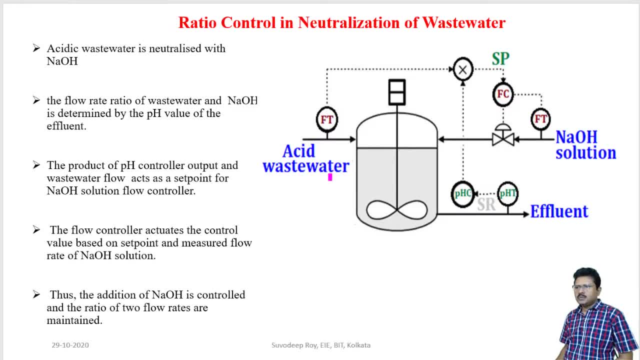 value of the effluent. This is the waste water. Before exposing it into the river or atmosphere, it is normally treated to maintain a particular pH value of that. To maintain that specific pH value, sodium hydroxide solution is normally added with the acidic waste water at a particular ratio. 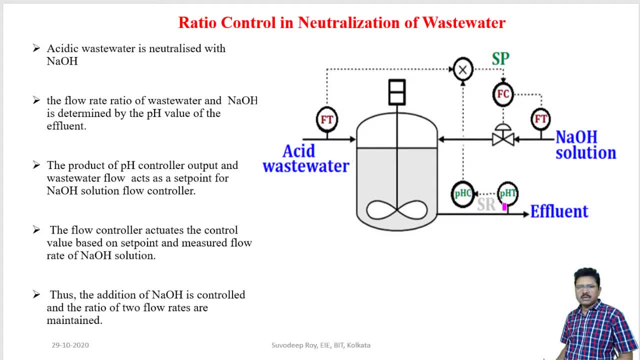 In this case, the pH of this exit effluent is normally measured and corresponding value acts as a ratio R. This is flow of acidic waste water, So this flow will be multiplied with the ratio R and this will be just like R into A, which is the set point for this flow controller, This flow. 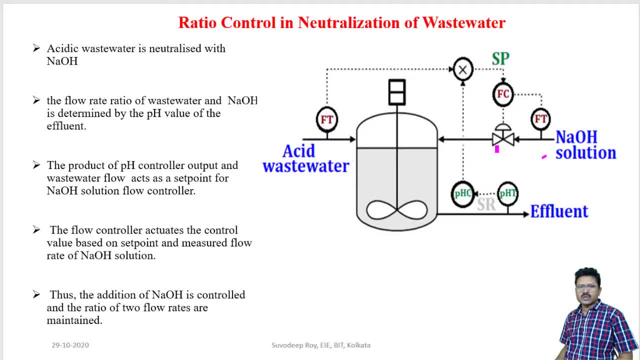 controller is used to control flow of sodium hydroxide solution. This flow transmitter is used to measure the flow rate of sodium hydroxide solution, This set point, which is coming from the value of pH, as well as the flow of acidic waste water According to the set point, and. 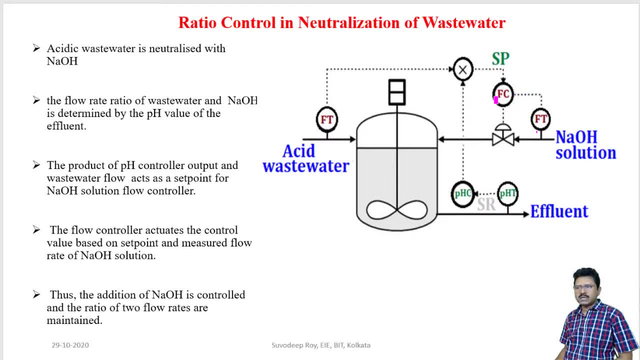 this process variable. this flow controller will produce a particular signal, This operates this control valve and ultimately control the flow of the sodium hydroxide solution to maintain the ratio between acetic waste water and sodium hydroxide with a particular value, So that, ultimately, pH value of the effluent will be maintained at a particular value, which is 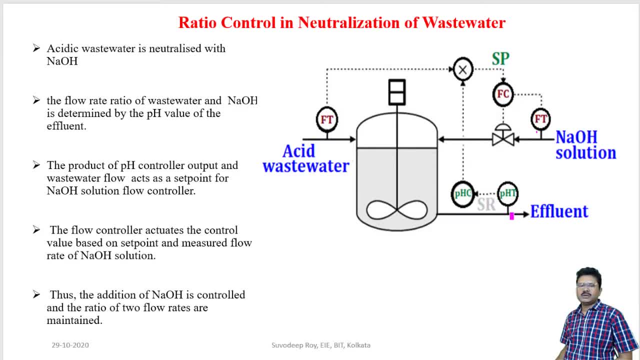 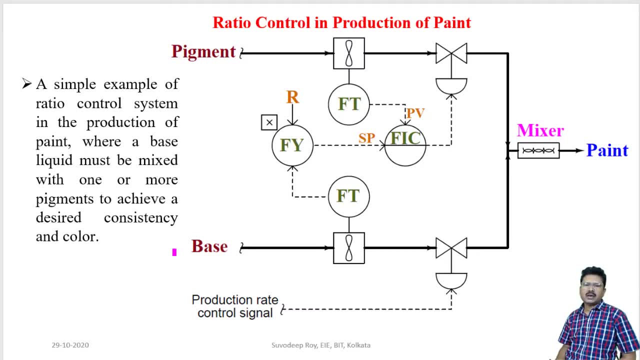 acceptable. So this is one example of ratio control system which is used to neutralization of waste water. There is another simple example of ratio control of sodium hydroxide solution, which is used to neutralization of waste water control system in the production of paint, where a base liquid must be mixed. 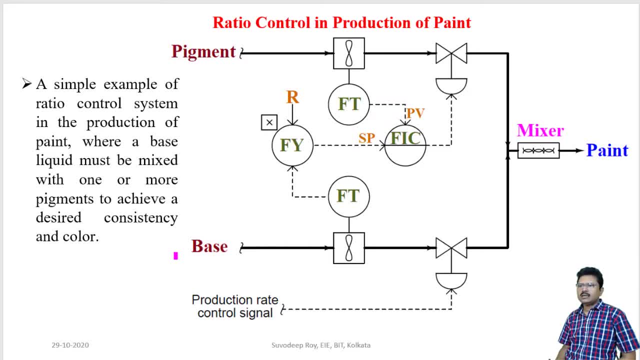 with on or more pigments to achieve a desired consistency and color this base liquid. this base liquid will be added with pigment at a particular ratio to get the particular consistency and particular color. flow rate of this base liquid is measured by this flow transmitter. so at this position this is: 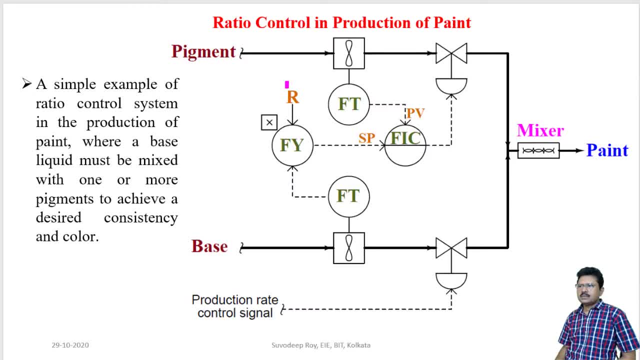 signal corresponding to flow rate of base liquid. this is the set point, which is R is the desired ratio. this R will be multiplied by this base liquid flow rate. ultimately, we will get a particular value which is just like R a. already we have explained this is the set point of this flow indicating controller, which 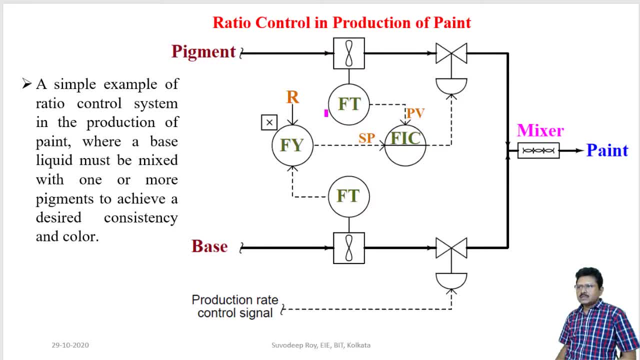 ultimately control the flow rate of pigment. this flow transmitter measures flow rate of pigment. so this is the process variable. according to the value of this process variable and the set point, the flow indicating controller will produce an output which ultimately operates this control valve. by operation of this control valve, the flow rate of the 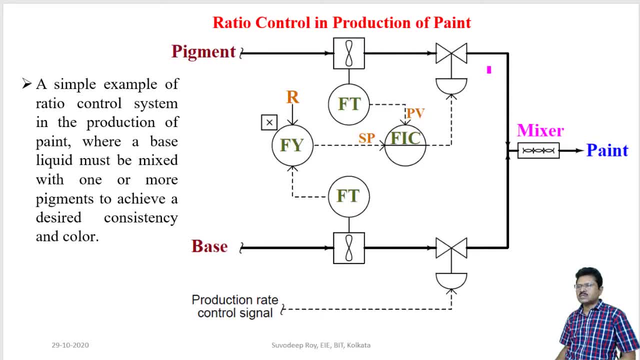 pigment will be maintained at a particular value so that, ultimately, there will be a specific ratio between this pigment and base at the mixer. when the specific ratio is maintained inside the mixer, a particular quality of paint will be produced with a specific color. this is one of the very simple. 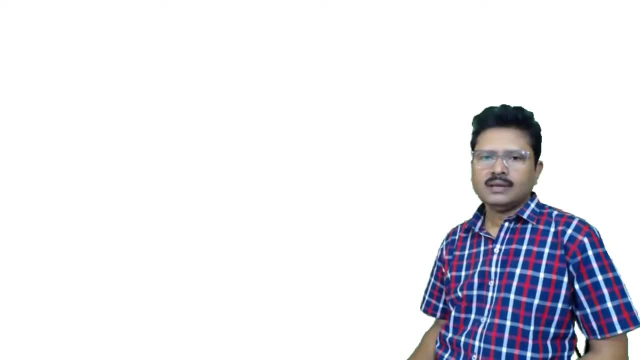 example of ratio control system in paint production in next tutorials. I will discuss this in the next tutorials. I will discuss this in the next tutorials. I will discuss in another techniques which are used in process control system. please put your in another techniques which are used in process control system. please put your. 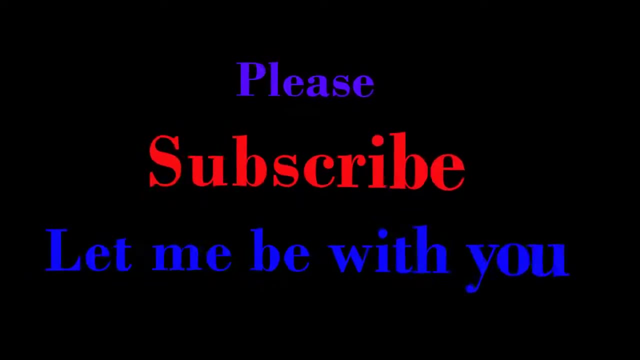 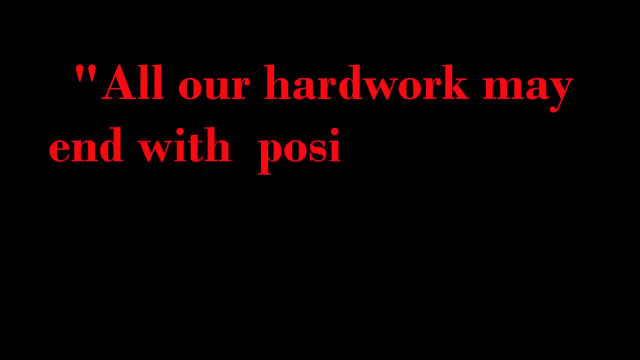 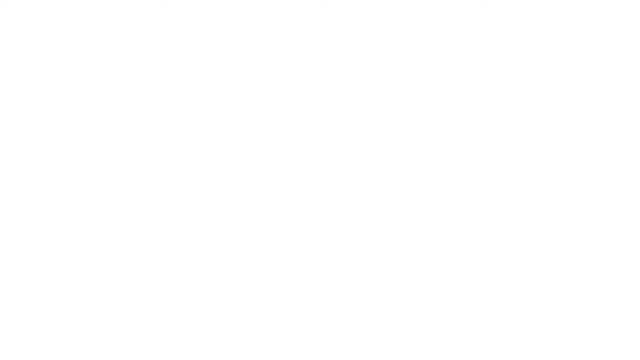 comments and suggestions in comment section in another techniques which are used in process control system. please put your comments and suggestions in comment section.